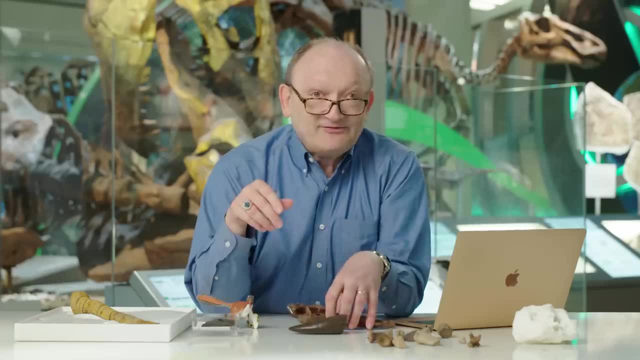 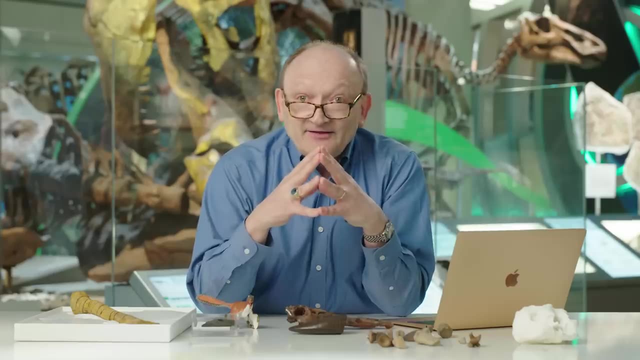 looked too puny and they needed something bigger. Strangely enough, shortly after this was filmed, people found a really gigantic raptor out in Utah, And since then other giant raptors have been found in South America and in Asia. So there were giant raptors around, but they were in fact much bigger. 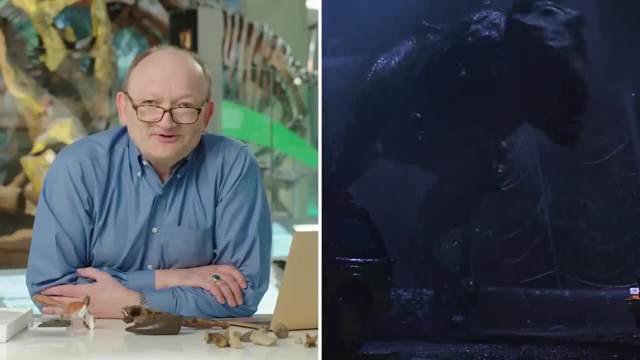 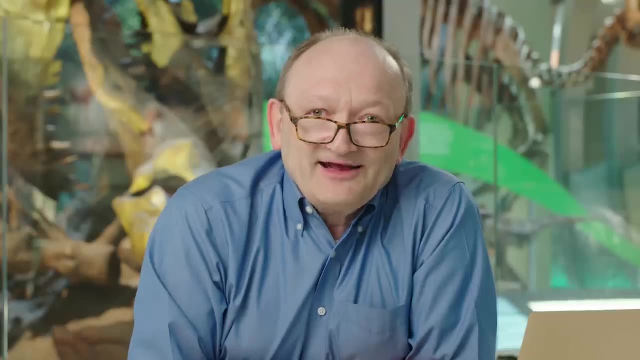 than the ones we saw in the movies, And so they were able to find a giant raptor in South America and the ones in the movie. The movie claims that T rex could only detect prey by motion. In fact, when we study the brain case of a T rex, we find that it had very large olfactory bulbs which are 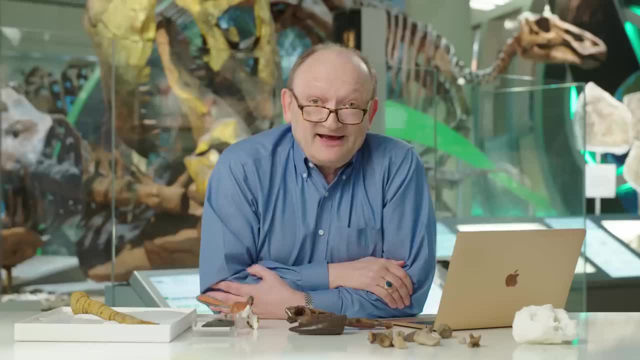 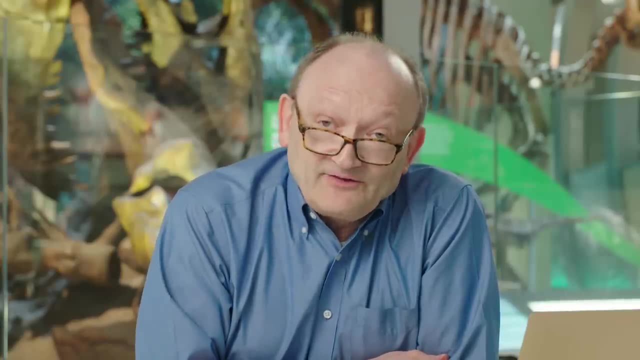 the part of the brain that picks up information from the nose. It had a very large opening for the optic nerve, which is the nerve that transmits information from the eye to the brain, And it had a very complicated inner ear that allowed it to hear at least a wide range of low-frequency sounds. 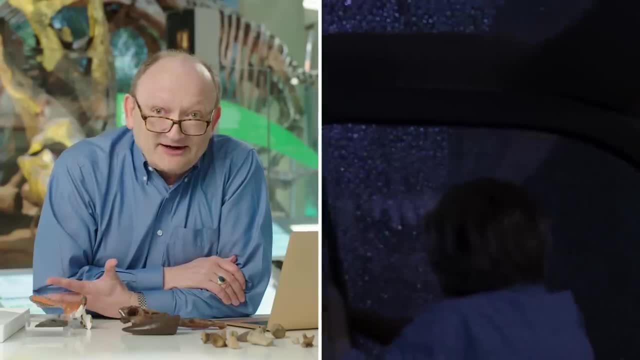 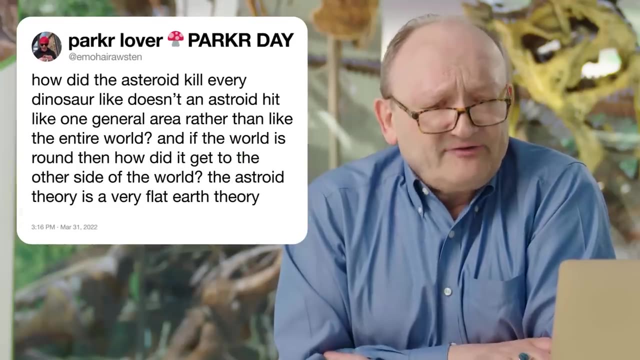 So it would have smelled like a raptor. but it wouldn't have been able to smell like a raptor. It would have smelled the actus in front of its snout and it would have been a very short movie indeed. Ed Emo, here a Western. How did the asteroid kill? every dinosaur Like 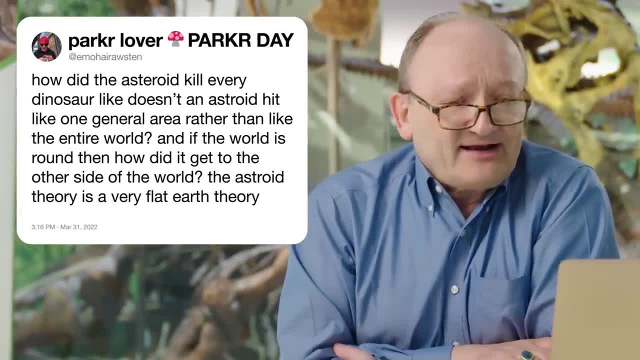 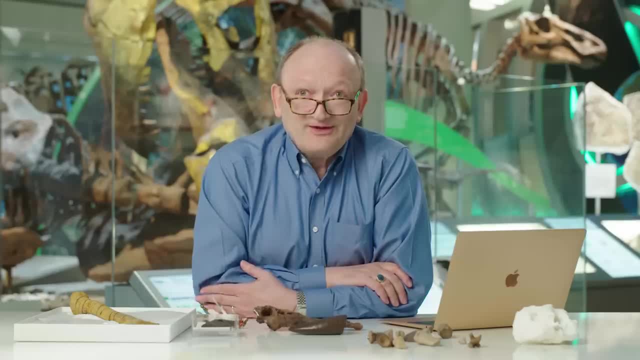 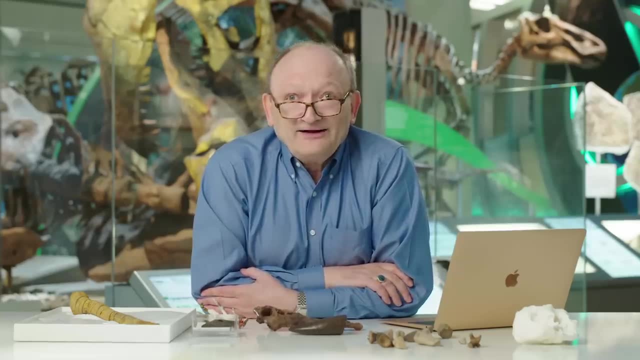 doesn't an asteroid hit like one general area rather than like the entire world? The asteroid theory is a very flat earth theory. There's no flat earth. The earth is a sphere. What happened was when the asteroid happened to impact, it released the equivalent of a hundred million. 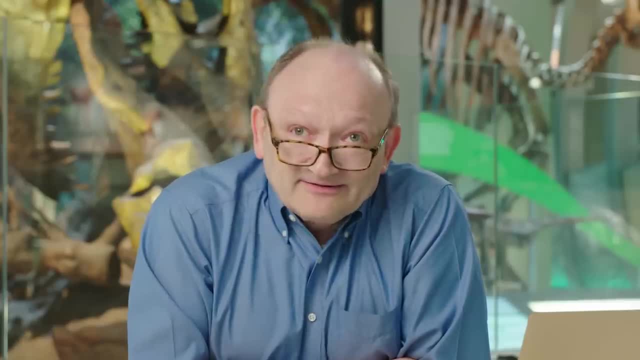 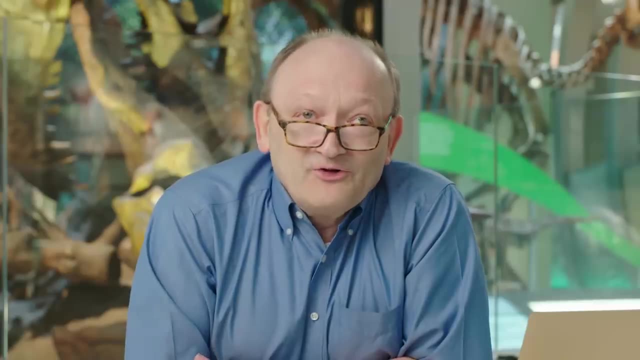 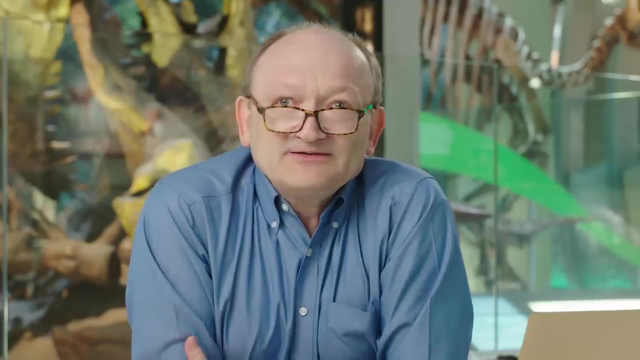 megatons of energy, And this basically melted this huge asteroid, which was six miles in diameter, And this sent up a gigantic cloud of glowing material up into the atmosphere. This would spread around the world. We see this even today when a volcano erupts. 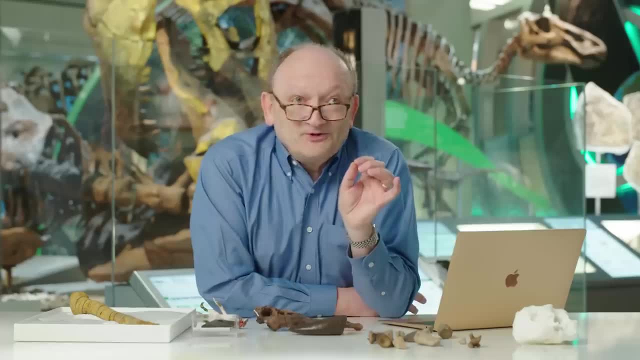 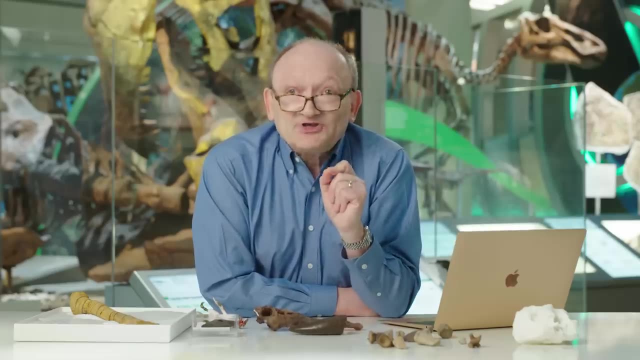 Volcanic dust sweeps all around the world. Imagine a world where suddenly it's raining drops of molten glass. That's what was happening, And so basically every larger animal at that point died. And that's what happened, And so basically every larger animal at that point died. 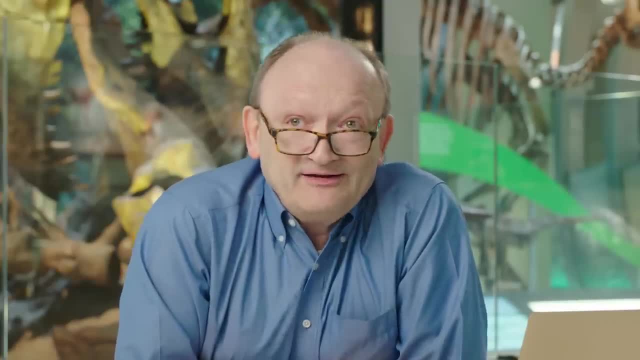 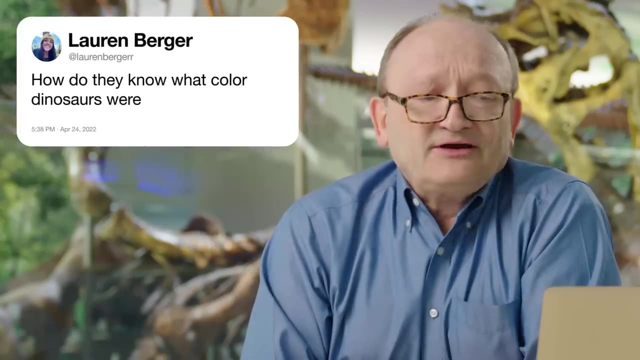 And that's why the dinosaurs were wiped out, probably within a matter of hours, at most a matter of days. Ed Lauren Berger asks: how do they know what color dinosaurs were? For many years, we really had no idea what color dinosaurs had. In fact. 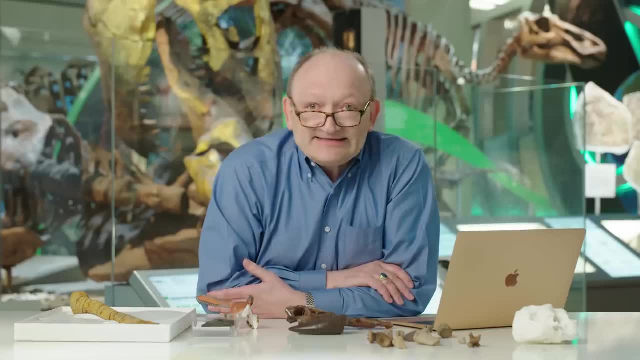 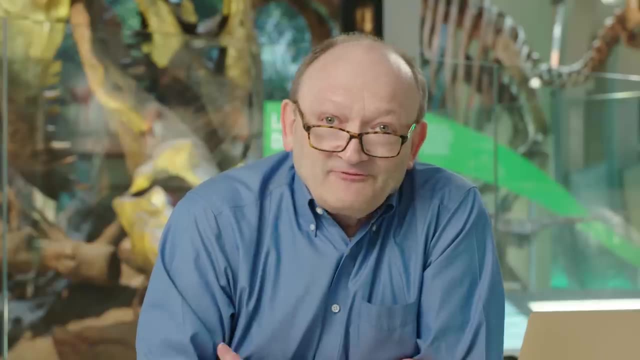 people sort of assumed that, like many of the modern lizards, snakes, crocodiles, turtles, it would have been sort of greenish brown, And that's what you see in all the old dinosaur books. However, in recent years, thanks to some remarkable discoveries in China, 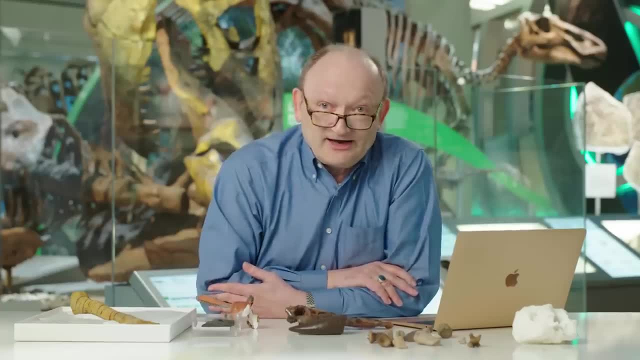 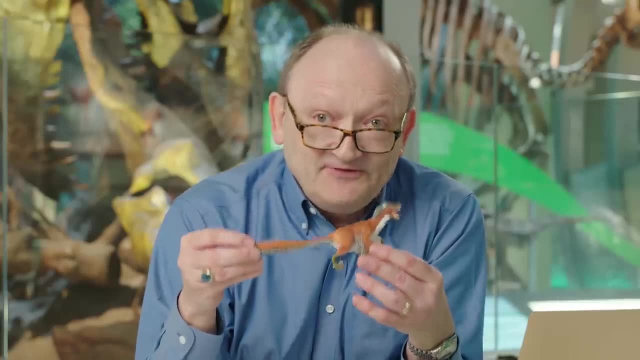 we actually found out what some dinosaurs looked like, And it was a real revelation. We found that some of the little feathered dinosaurs actually had color patterns as vivid as those in modern birds. There's a dinosaur called Cao Long and it had beautifully. 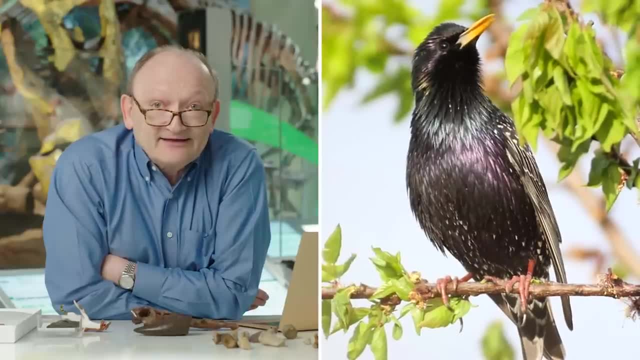 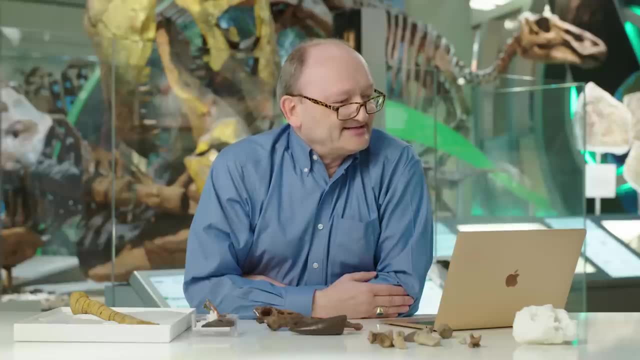 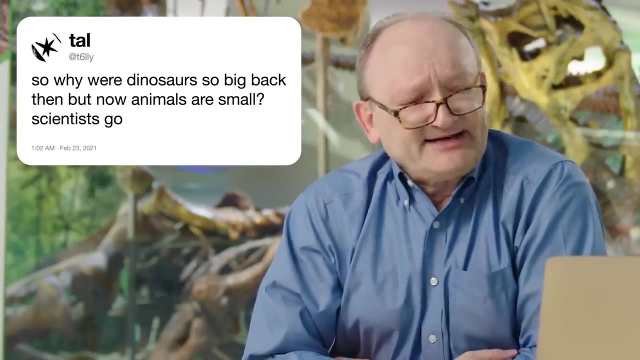 iridescent feathers. So it would have looked like a big starling with nasty claws. So the dinosaur world was far more colorful than we were previously thinking At T6. Lee asks: so why were dinosaurs so big back then? but now animals are small, Scientists go. A lot of dinosaurs were big, but there were also small dinosaurs. In fact, there's one dinosaur that's barely over two feet long. Do you live in an environment where it's advantageous to be big for your particular mode of life? And there are some places on earth where the rules are reversed. 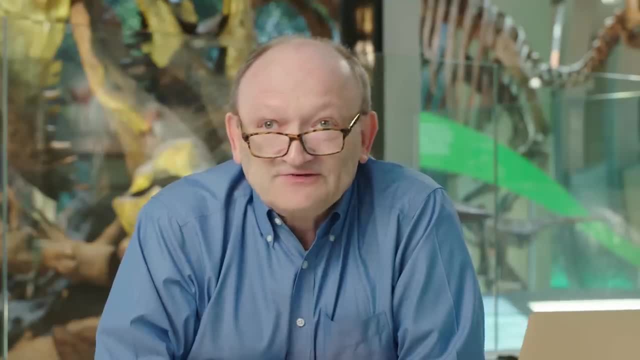 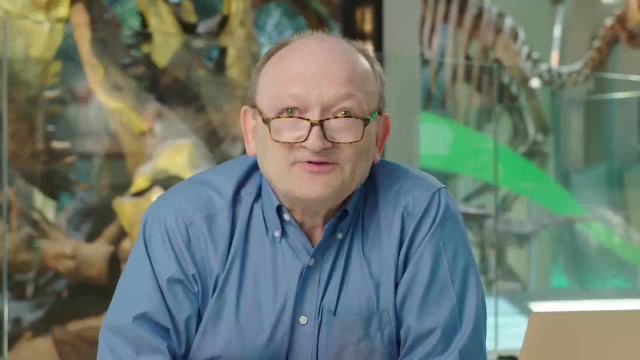 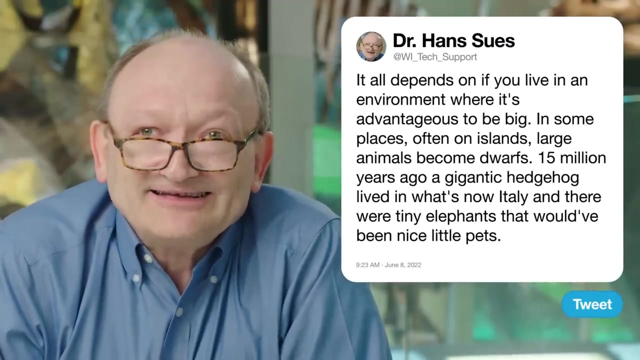 Often on islands. generally large animals become dwarfs. About 15 million years ago a gigantic hedgehog lived on an island in what is now Italy. In other parts of the Mediterranean there were tiny elephants running around. They would have actually sort of been nice little pets if we had been around at that time. 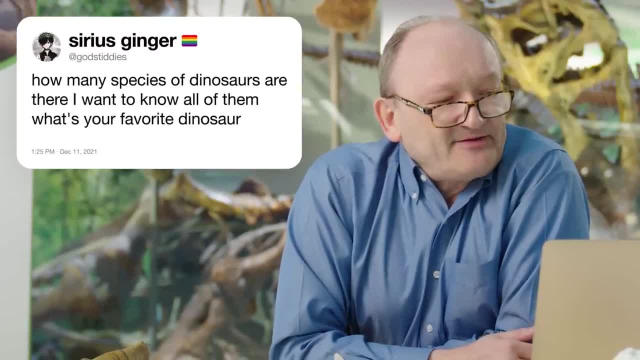 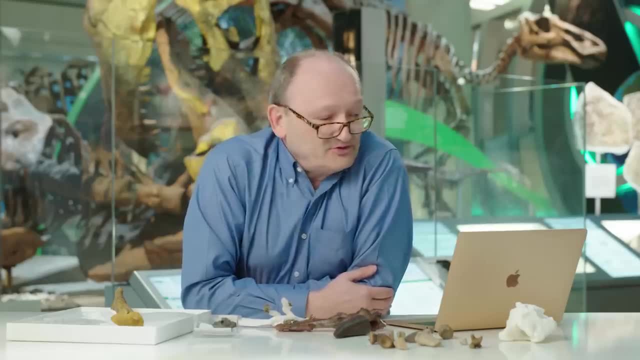 God Stiddies asks how many species of dinosaurs are there? I want to know all of them. Right now there are about 1,100 described species of dinosaurs other than birds. Even very conservative estimates put the number much higher, anywhere between 2,000 and 5,000.. 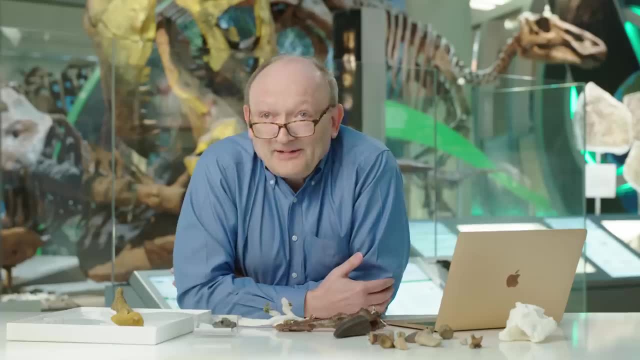 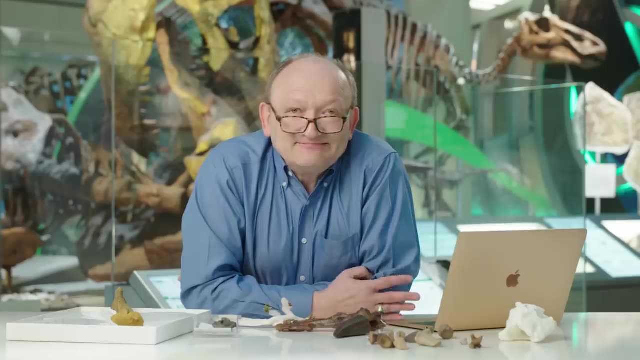 And there may have been even more. One important thing to keep in mind is we are much closer in time to a T-Rex than the T-Rex was to a Stegosaurus. We now have classified this myriad of species by looking at various parts of their skeleton. The most obvious part of 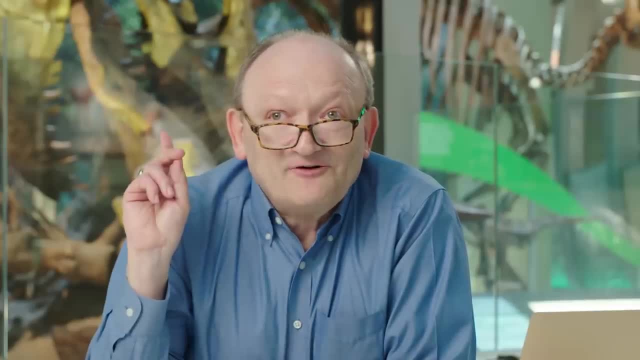 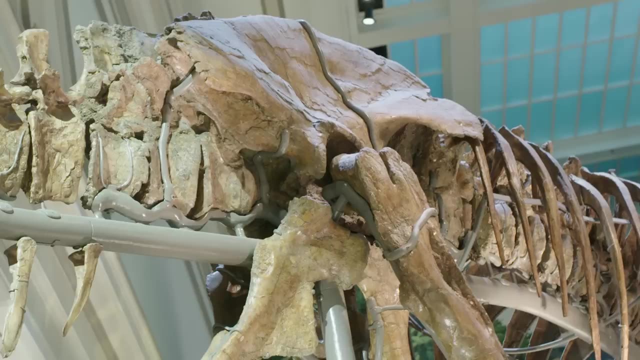 the skeleton is the hip region. When you look at the T-Rex over my shoulder here, you can see a hip girdle that has three bones, with the front bone, the pubic, pointing downwards, whereas in the so-called bird-tipped dinosaurs, which is unfortunately misnomer, since they have 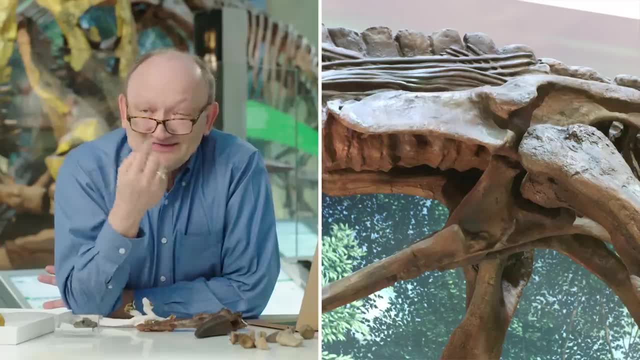 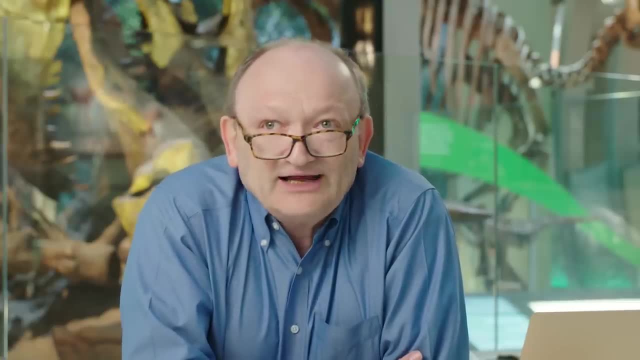 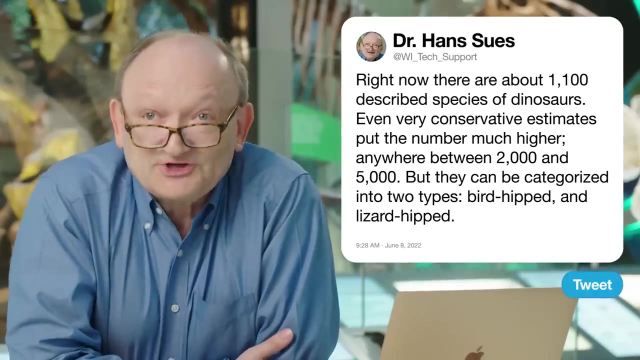 nothing to do with birds. You get a hip region that has the pubic bone pointing backwards. There are many more subtle anatomical differences, but basically there are two large groups of dinosaurs: the lizard-tipped dinosaurs, also called Saurischia, and the bird-tipped dinosaurs called Ornithischia. 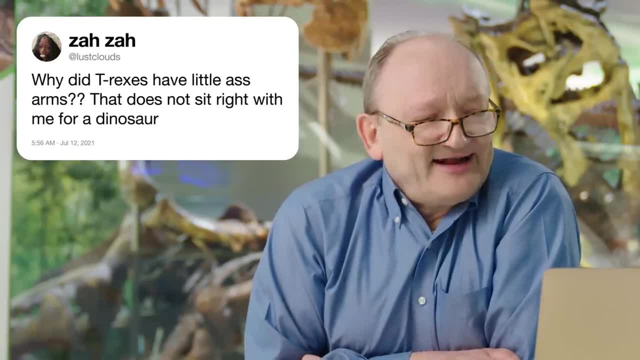 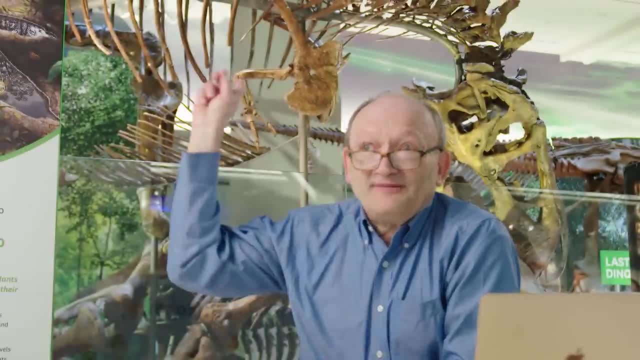 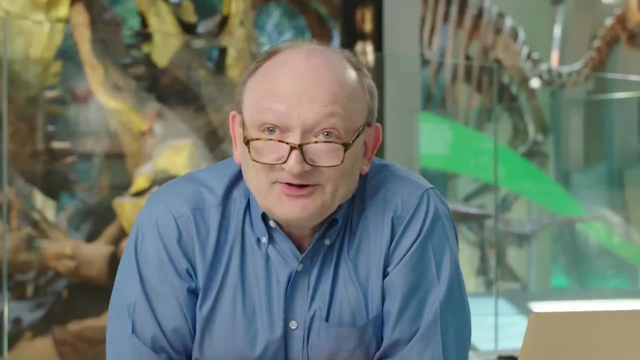 At Lust Clouds asks: why did T-Rexes have little-ass arms? That does not sit right with me for a dinosaur. T-Rex had really small but very powerful arms, and you can see this here on our pride and joy. Nobody really knows why T-Rex has tiny arms. It has been calculated that the arms were still strong enough to lift up to 600 pounds of weight. Earlier relatives of T-Rex still have longer arms. Other predatory dinosaurs actually get increasingly longer arms, which eventually become wings in birds. Add solar wings us. Since when were pterodactyls not dinosaurs? Since ever Dinosaurs and pterodactyls are. 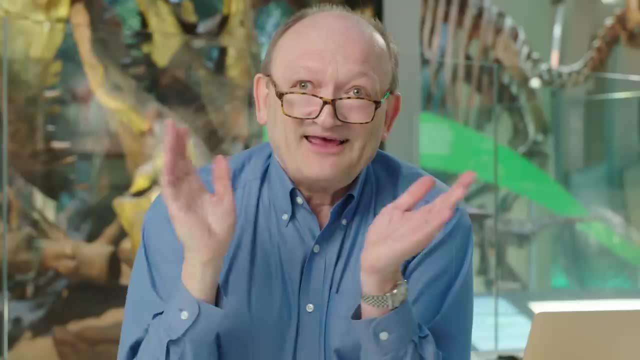 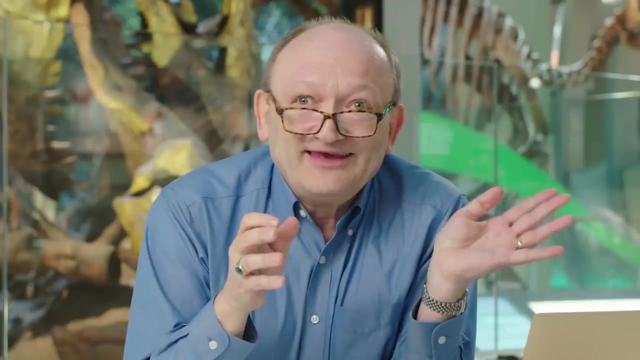 related but pterodactyls have nothing to do with dinosaurs. They have an early common ancestor but they diverged in their evolution quite dramatically. Pterodactyls became flying creatures, wings very different from those of birds. Of course, dinosaurs were mostly. 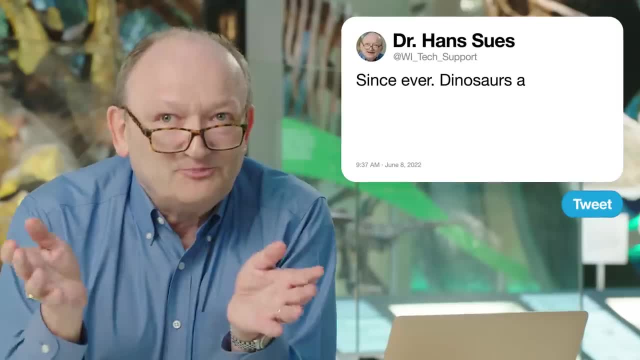 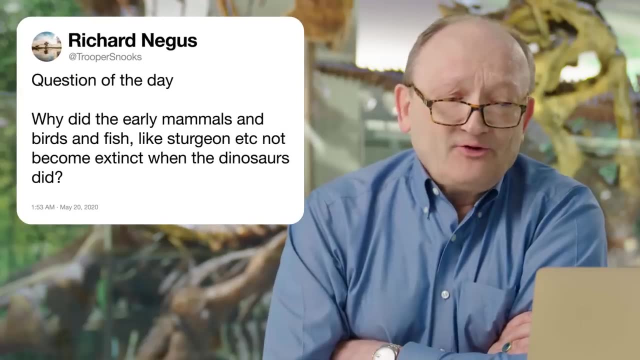 land-dwelling animals and only a few forms later on evolved into birds which have very different-looking wings. At Trooper Snooks asks the question of the day. why did the early mammals and birds and fish like sturgeon, et cetera? not have wings? Why did the early mammals and birds and fish like sturgeon, et cetera, not become extinct when the dinosaurs did? That's a very good question and in fact it's one of the great mysteries of paleontology. It's basically different life strategies Small animals can hide. 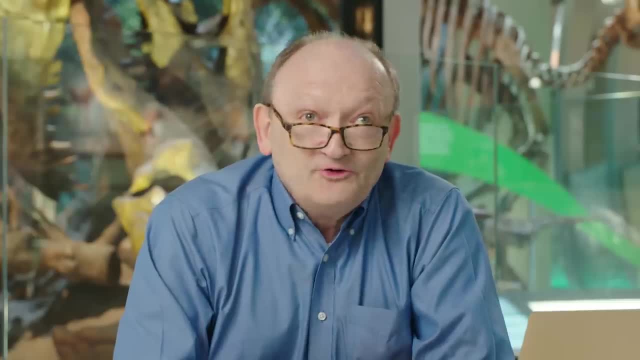 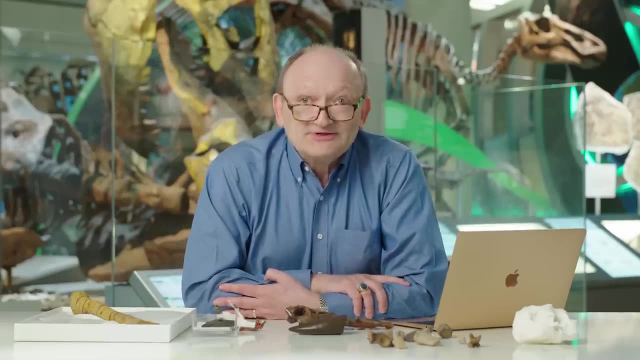 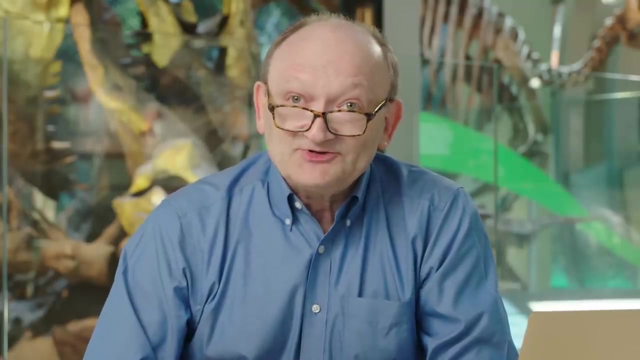 A lot of small animals are also able to go without food for long times, whereas a large animal cannot. Most dinosaurs went extinct and only one group of dinosaurs- birds- survived. Birds, as I just said, are dinosaurs because they descended from small, meat-eating dinosaurs, just like we are. 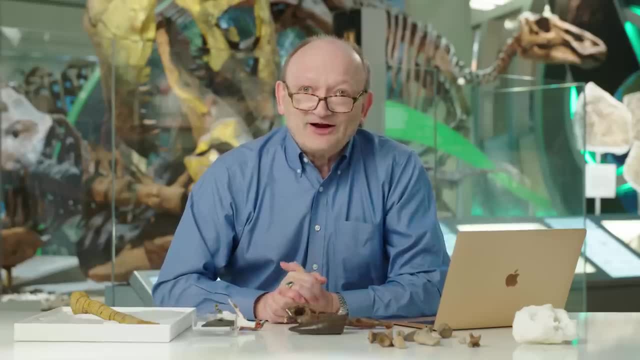 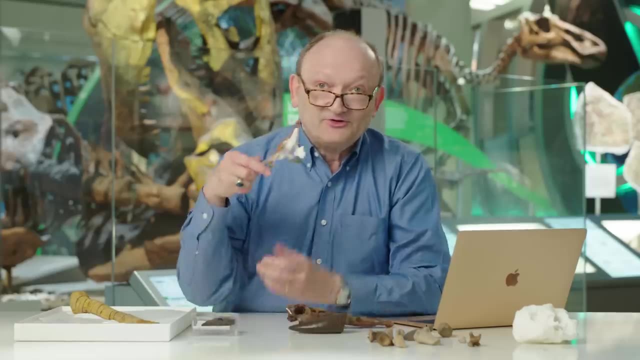 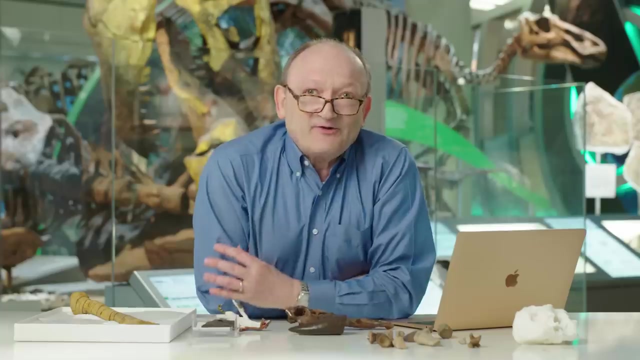 primates because we descended from other kinds of primates. We now have a beautiful series of fossils documenting all of the stages between little predatory dinosaurs like that and birds that would have been recognizable as a bird to anyone alive today. It's very rare that you get. 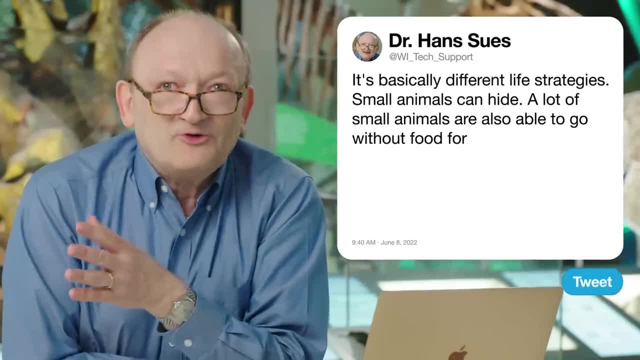 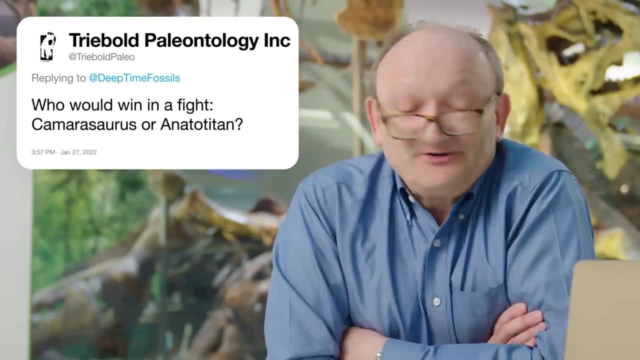 such a nice continuation of fossils between one group and a group that it gave rise to, At Trebow, to Paleo. who would win in a fight? Camarasaurus or Anatotitan? Anatotitan and Camarasaurus lived at very, very different points in time. Anatotitan at the end of the. 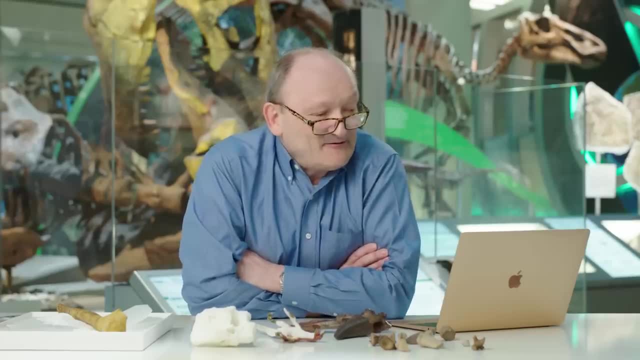 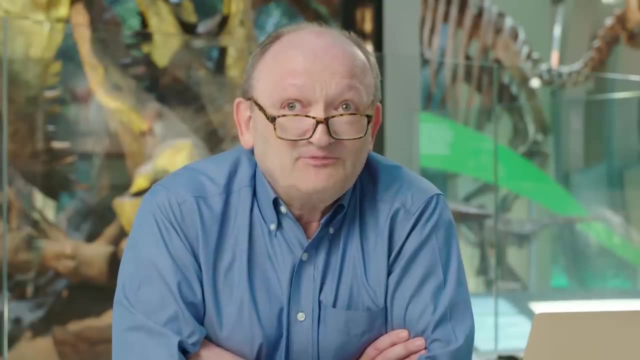 Cretaceous period about 66 to 68 million years ago, and Camarasaurus about 150 million years ago. My money would be on the Camarasaurus, simply because Camarasaurus got a lot bigger. Both, however, were harmless plant eaters, and so I don't think they would have really fought each other. 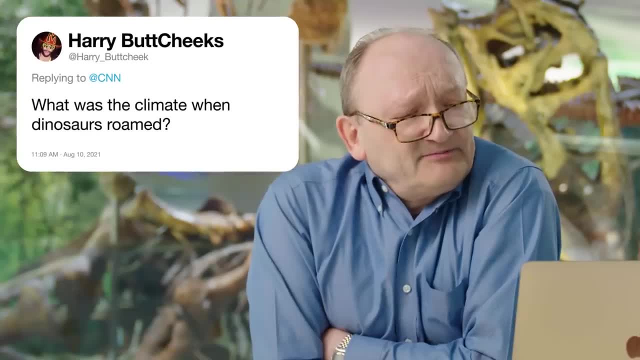 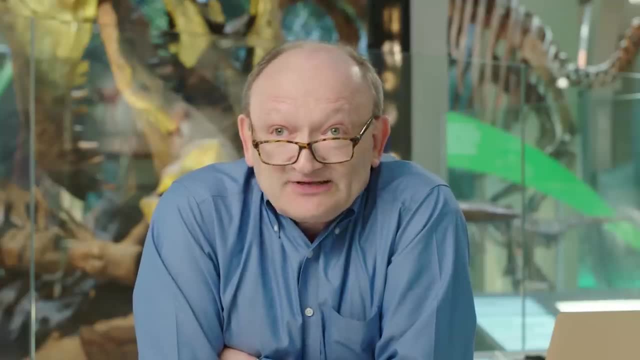 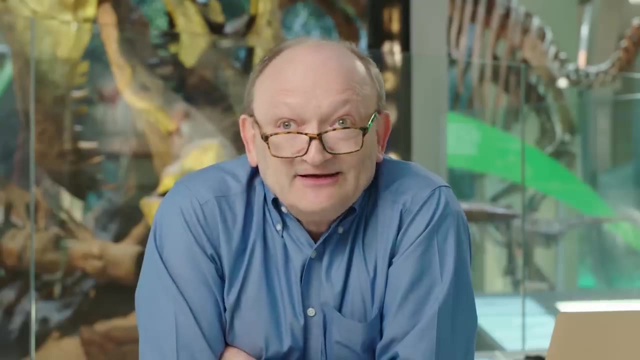 At. Harry Buttcheek asks: what was the climate when the dinosaurs roamed? The world in which dinosaurs lived was generally a fairly warm warm one. However, at high latitudes, where the sun would disappear for months at a time, it would have been quite cold, and we actually have even evidence from fossil soils that there 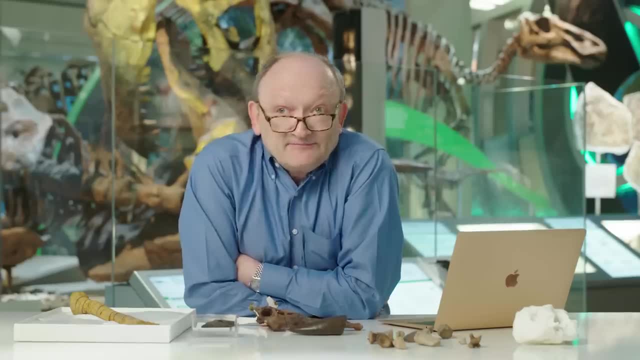 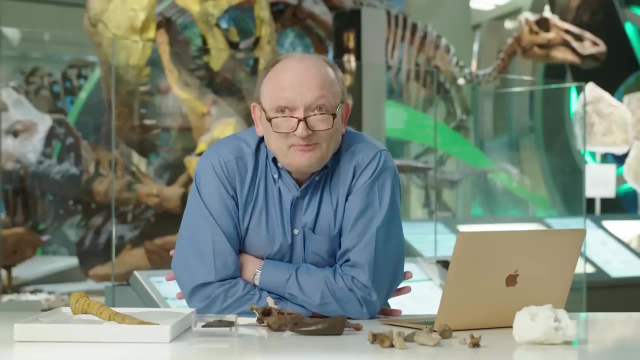 were permafrost soils in some areas, Yet dinosaurs lived there. Dinosaurs really could cover almost any environment that you can imagine. We know dinosaurs that lived essentially under subpolar conditions. We know dinosaurs that lived in really tropical regions. We know dinosaurs. 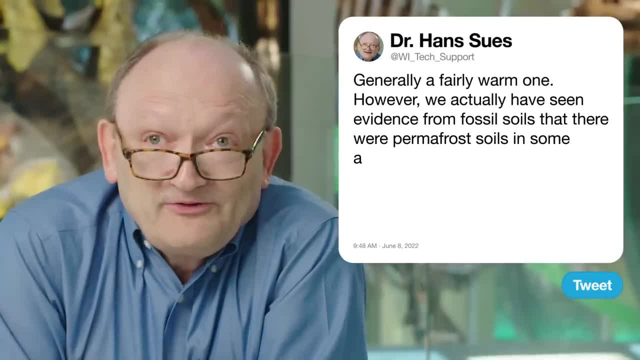 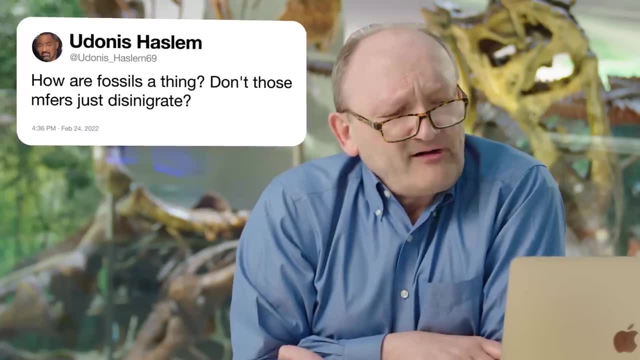 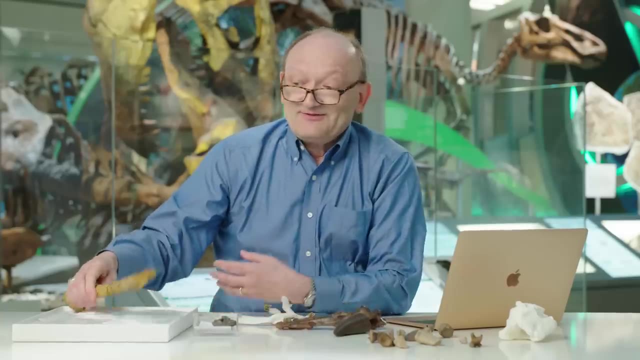 that lived in deserts. So basically, in a warm period of geological history, they were everywhere. At Eudonis, Haslam 69 asks: how are fossils a thing? Don't those people just disintegrate? Well, fossils are a thing. They're real three-dimensional objects. 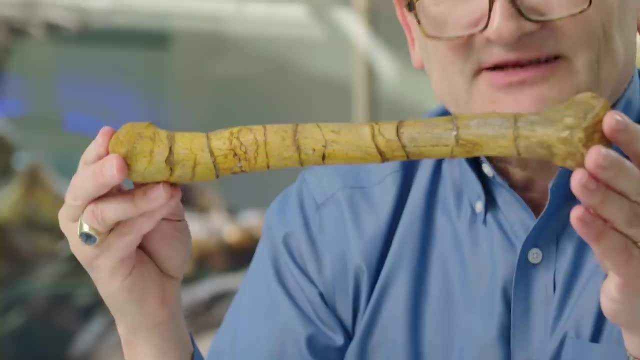 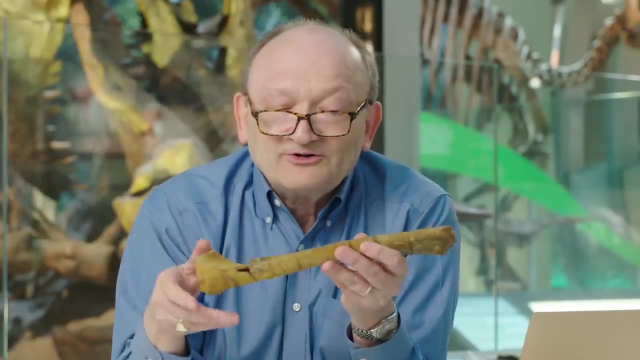 Here's a limb bone of an ostrich mimic dinosaur that's about 90 million years old. Basically, what happens is, after death, minerals infiltrated this bone from the groundwater around it and they contained a lot of iron. That's why it has this yellowish-brown color And gradually, 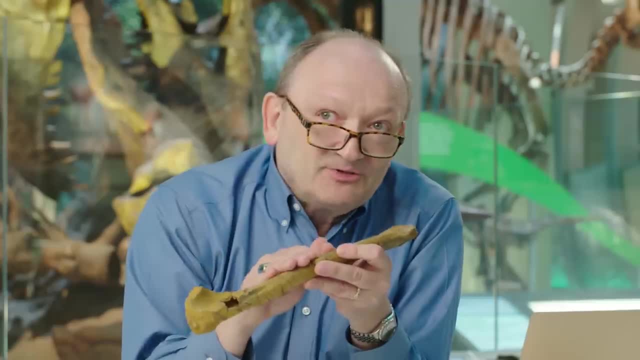 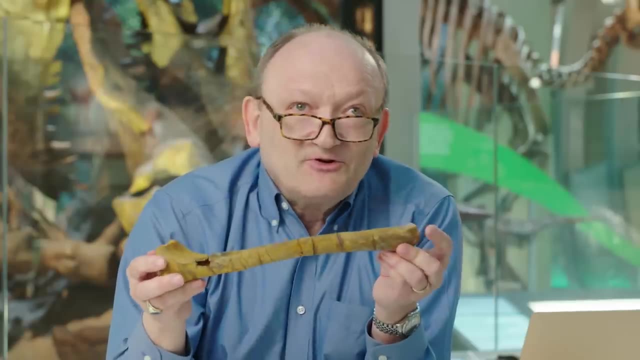 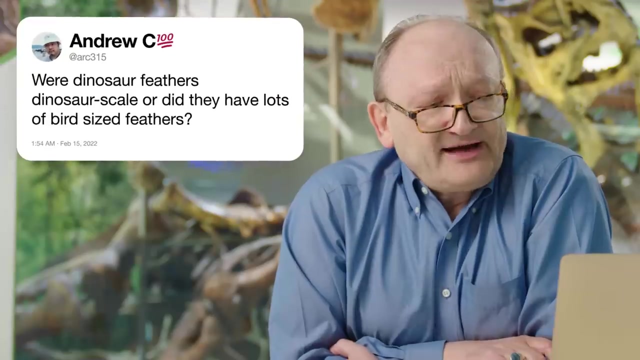 filled in all of the spaces in the bone. Sometimes the actual bone is still pretty much preserved, but in most cases the bone has changed just ever so slightly so that it's no longer possible, for instance, to extract biomolecules like DNA from it. Ed Ark 315 asks: were dinosaur feathers? dinosaur scale or did they have a lot of bird-sized feathers? The really gigantic dinosaurs by and large did not have feathers. We only know one really large tyrannosaur from China that lived in a very cold environment and had feathers. Most of the dinosaurs that we know that had feathers. 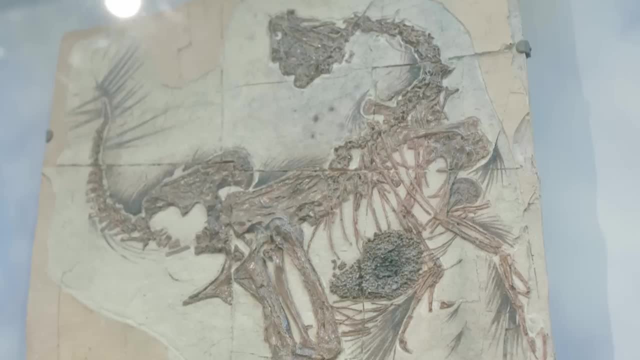 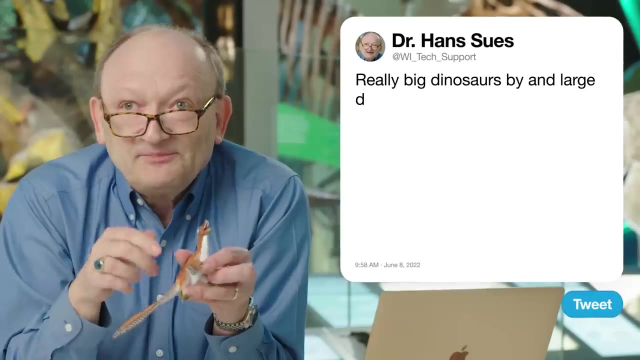 were animals up to maybe five or six feet in length and they had bird-sized feathers, And we know this because the bones have little bumps on them and you can see them when you take a chicken apart. They're called quill nodes and that's where the large flight feathers in a bird. 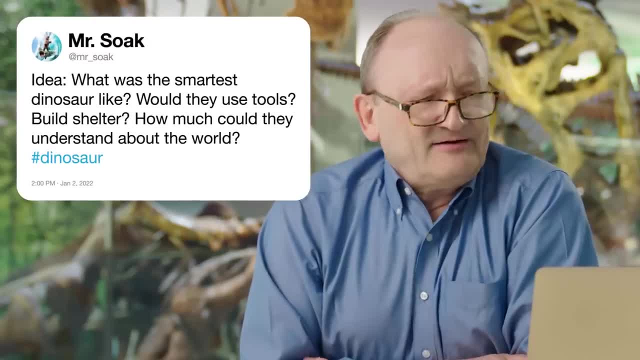 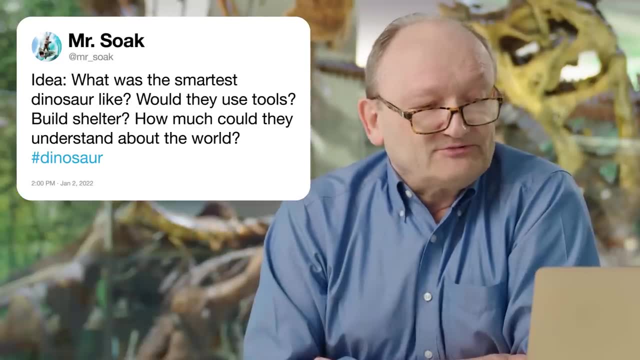 insert: Ed. Mr Soak asks idea: what was the smartest dinosaur like? Would they have used tools, built shelter? How much could they understand about the? How much could they understand about the? How much could they understand about the world? Some of these little predatory dinosaurs have really large brains. They have this sort of 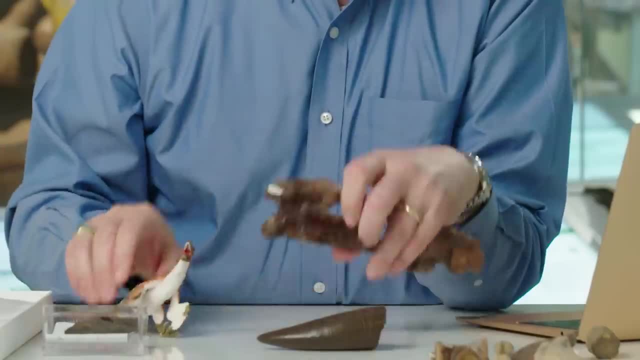 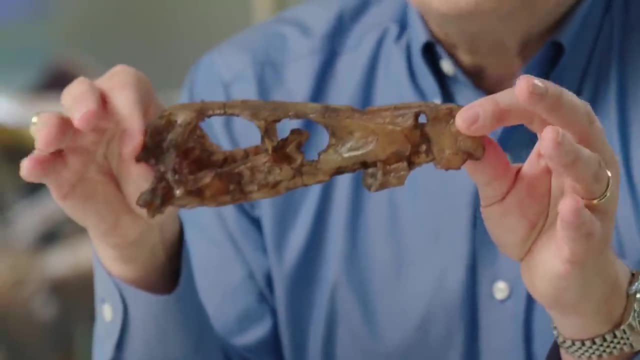 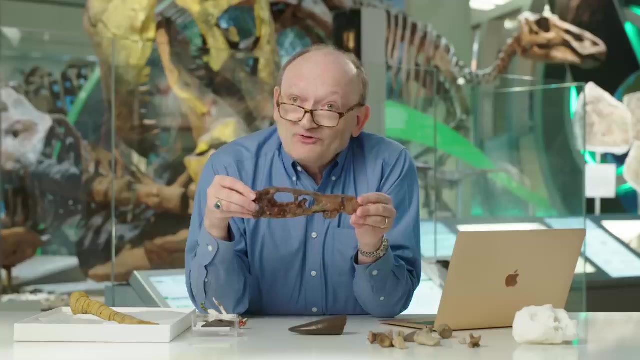 bulging area here, much like you would see on a bird skull. So these little dinosaurs probably had cognitive abilities similar to those that we see today in hawks, owls and particularly in crows and ravens. Crows and ravens have repeatedly shown their ability to solve relatively complex 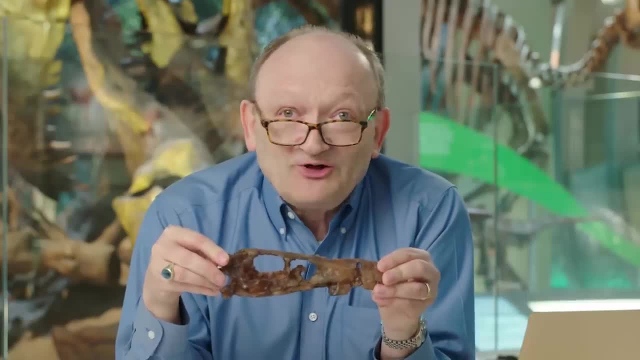 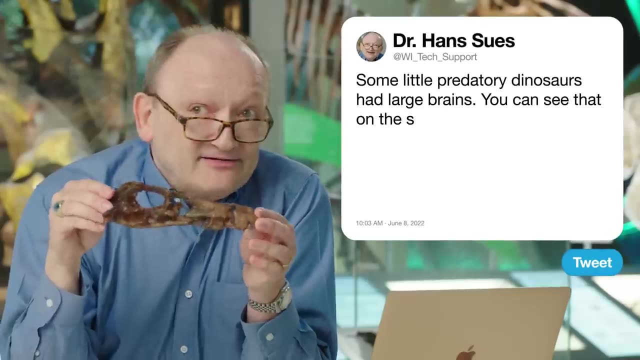 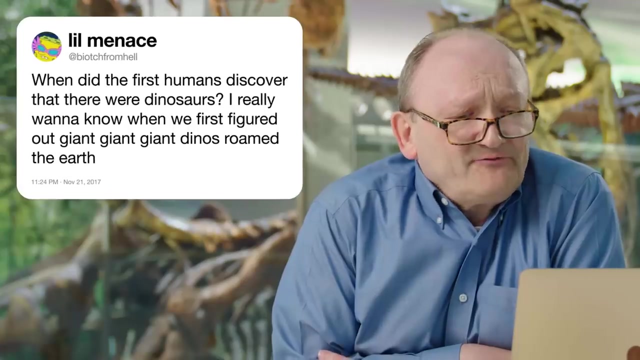 problems, and some birds have sort of made them more capable of solving relatively complex problems. They have sort of minimal kinds of tool use as well, and something like that is not beyond the possibility for these early dinosaurs as well. Ed Birch from Hell us. when did the first humans discover that there? 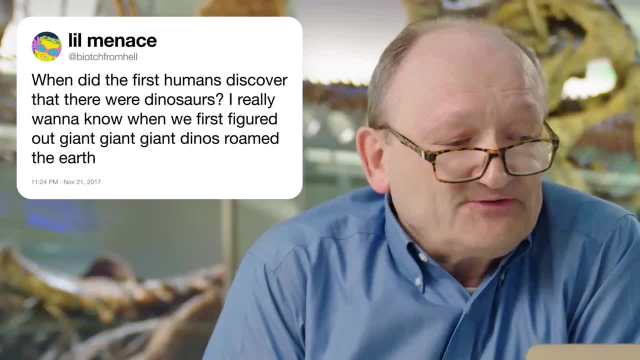 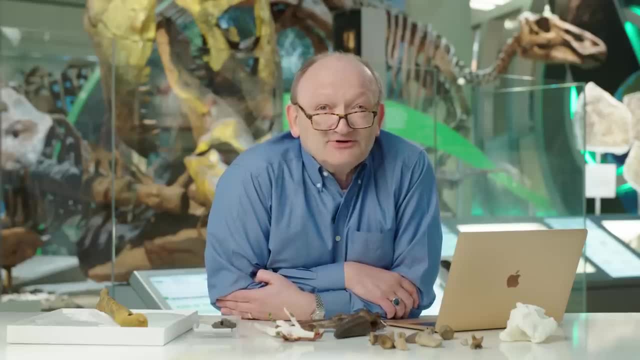 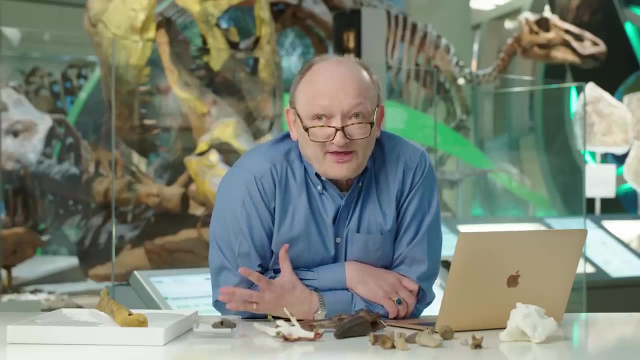 were dinosaurs. I really want to know how we first figured out giant, giant, giant dinosaurs roamed the earth. The first record that we know of a definitive dinosaur is from the 17th century in England, when Robert Plott described a part of a fiber-based 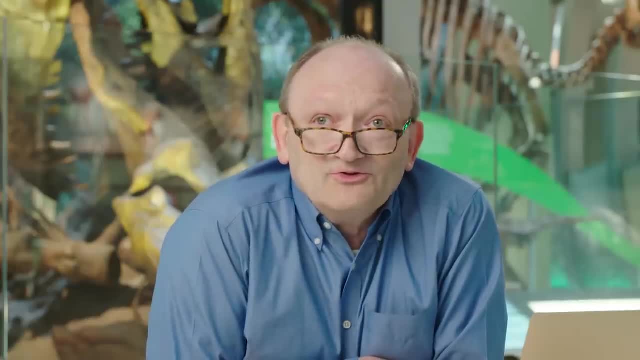 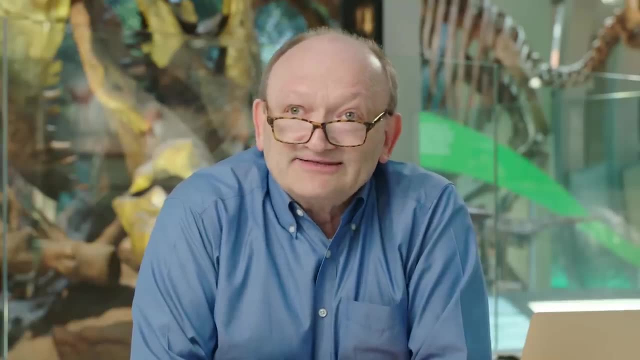 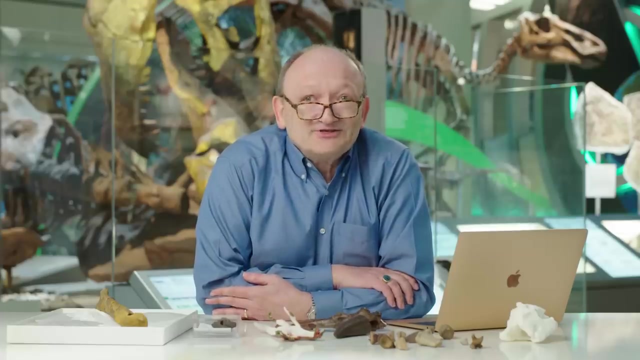 bone. He didn't know what to make of it. He compared it to giants of legend. President Thomas Jefferson couldn't conceive of the fact that animals had gone extinct. Even though he found fossils of extinct animals on his estate in Virginia, he thought that these animals still. 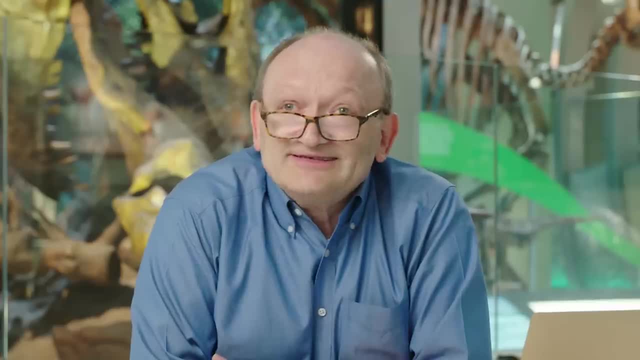 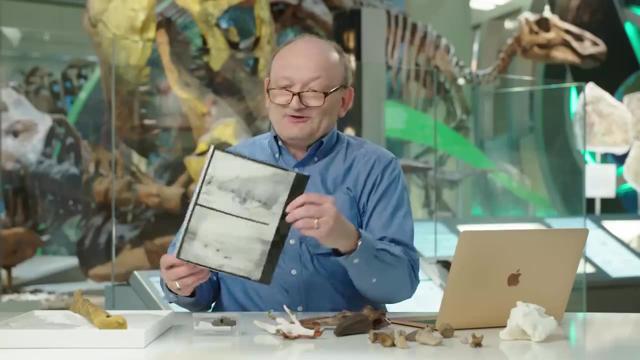 existed somewhere alive out west, and that was one of the reasons he sent the Lewis and Clark expeditions out. The Smithsonian got into the dinosaur business early in the 20th century and here's an old photograph. This one is from the 17th century and this one is from the 18th century. 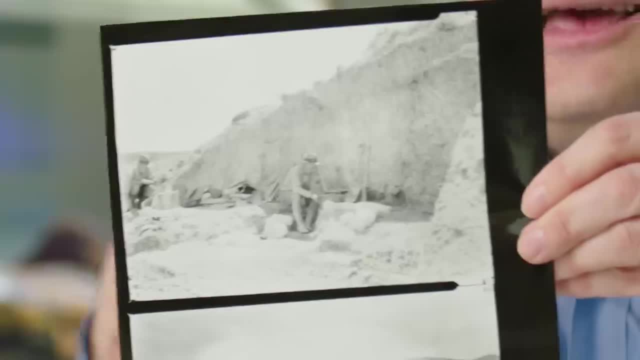 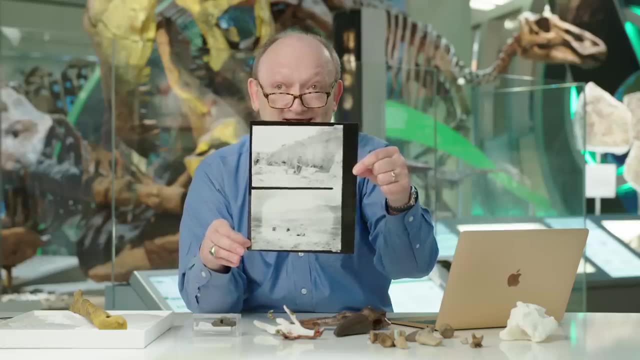 This one was taken in the 1930s- an excavation in progress, and you see people here chipping out large blocks of rock that have bone in them and then are taken back to the laboratory where the actual excavation begins. We can glue it back together, clean its surface and ultimately it's 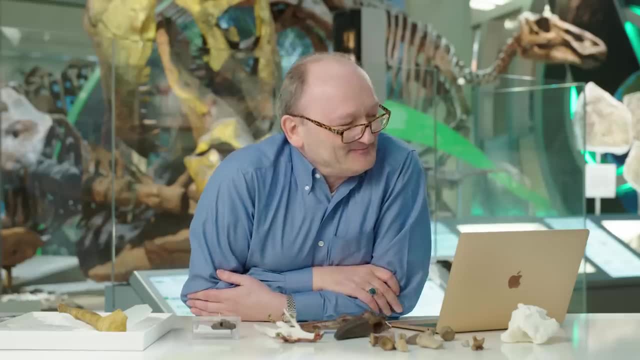 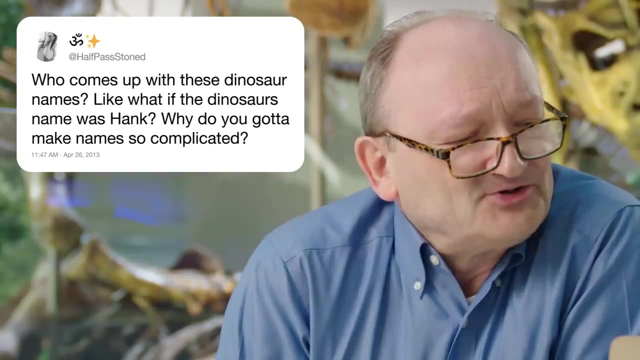 ready for study and exhibit. Ed Halfpast Stone us. who comes up with these dinosaur names? Like, what if a dinosaur were named Hank? Why do you got to make names so complicated? The scientists who described the dinosaurs come from the 19th century. They came from the 18th century and they 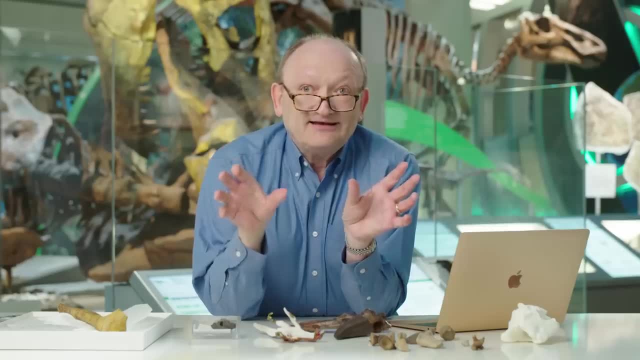 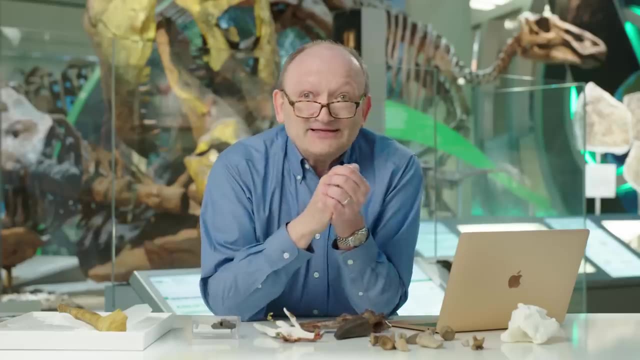 came up with the names. Each animal has a genus and a species name and in the case of dinosaur names it's the same: It's Tyrannosaurus rex. In that case, it's actually one of the best names ever chosen for a dinosaur, because the researcher wanted to portray it as the tyrannical creature. 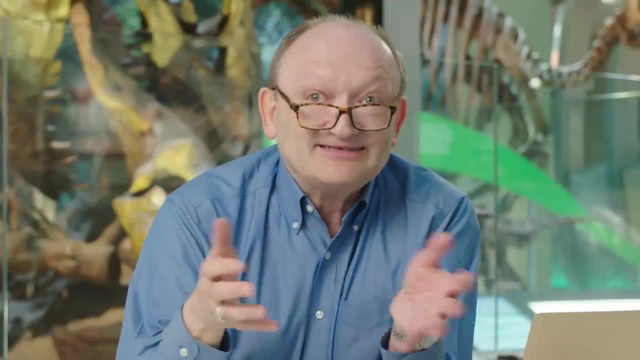 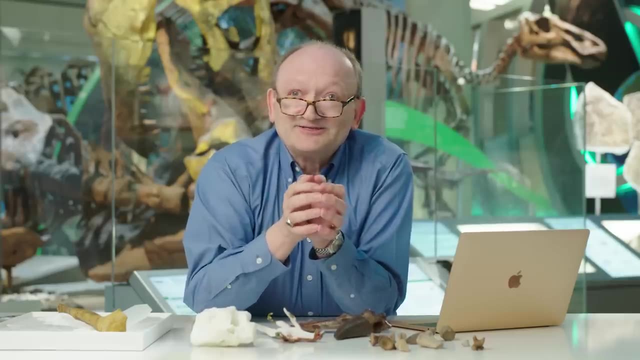 that ruled its ecosystem and because of its big size it's called rex, which means king. I've been very fortunate that somebody named the dinosaur for me. There's an animal called hansuthia, which is a little bone-headed dinosaur. 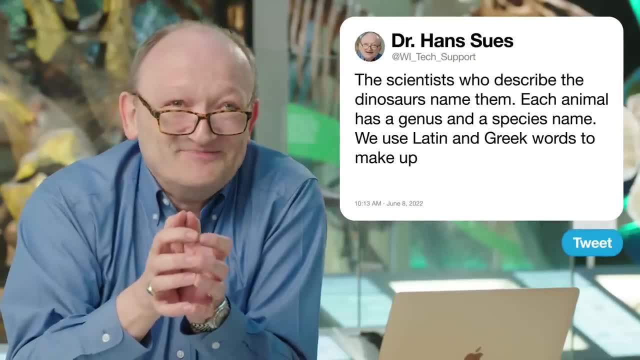 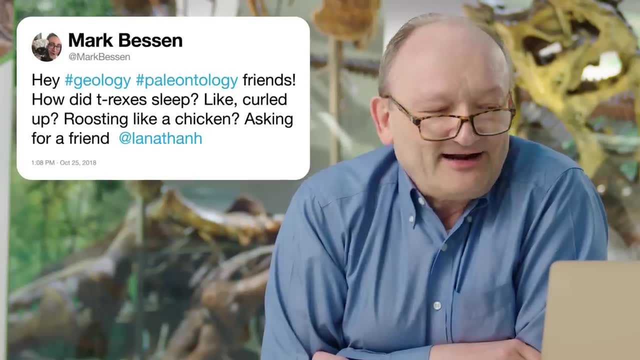 which I sort of take as a backhanded compliment that I'm bone-headed. But it's a nice thing because it kind of immortalizes you. Edmar Besson us: how did T rexes sleep Like curled up? roosting like a chicken asking for a friend. T rex presumably crouch down, just like a lot of birds do when they're resting. However, we actually have found dinosaurs that were preserved in burrows, where they presumably were sleeping or at least hanging out, and some of them are kind of curled. up. Ed Paul Garcia, us. who comes up with the name hansuthia is a little bone-headed but it's a nice thing because it kind of immortalizes you. Edmar Besson us. how did T rexes sleep Like curled up? at Paul Garcia NBA us. how did the brontosaurus weigh 23 tons when it only ate plants? You have to imagine that these dinosaurs probably spent every waking minute eating. The other reason that brontosaurus is so big is if you eat plants, you have a big problem. Much of 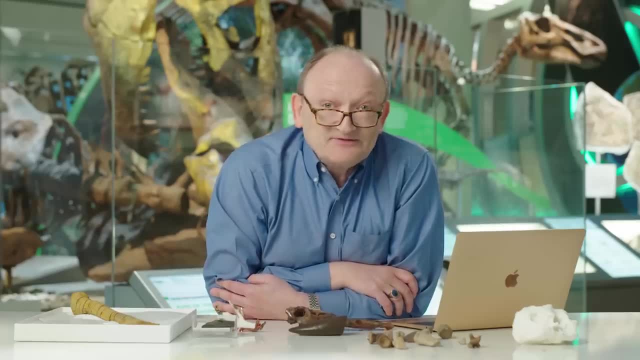 the plant food that animals and people eat is made out of cellulose, and so you need a very large gut to accommodate bacteria and other microorganisms that can break the cellulose down into fatty acids. So you need a very large gut to accommodate bacteria and other microorganisms that can break the cellulose down into fatty acids. 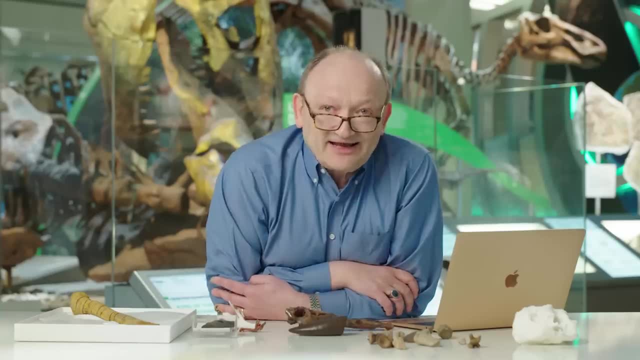 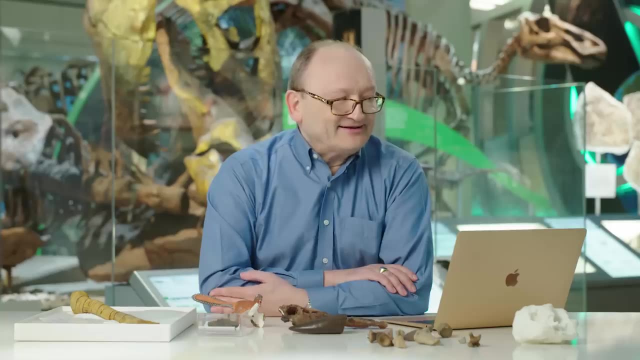 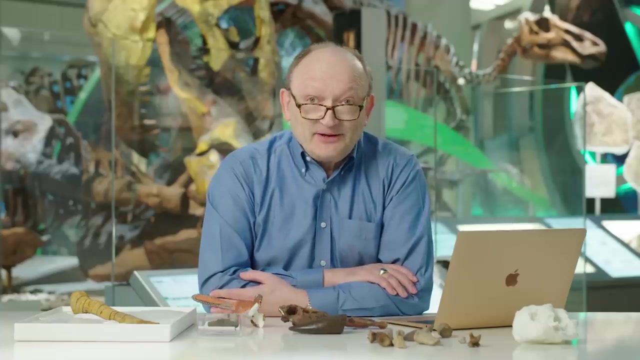 acids and in sugars like glucose, that the host animal can actually digest. So in order to be a full-time plant eater, you need a really large gut. Ed Allard Elagen us: were dinosaurs, cold-blooded or warm-blooded? I genuinely have no clue. Well, this has been a matter of scientific debate for 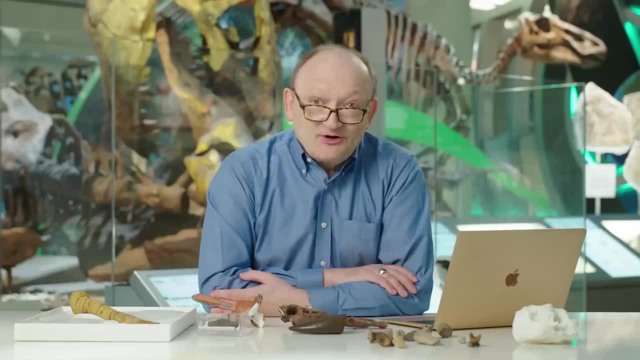 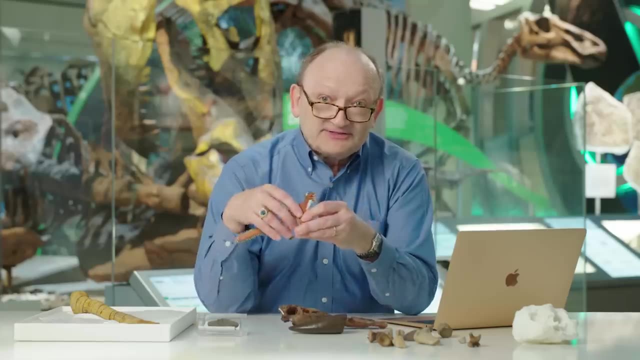 many years, but we now think that dinosaurs have a mixture of body temperature strategies. The little feathered dinosaurs were warm-blooded, much like the descendants birds, but some of the really large dinosaurs actually were either warm-blooded or cold-blooded, because when you have a really large body mass and live in a warm climate. it doesn't really matter either way. Ed Allard Elagen us: how long did the dinosaurs live for? Weren't they around for like a million years or something? Well, dinosaurs as a group first show up 230 million years ago. most dinosaurs went extinct. 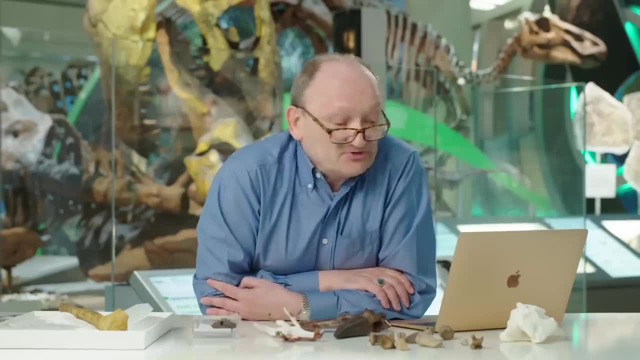 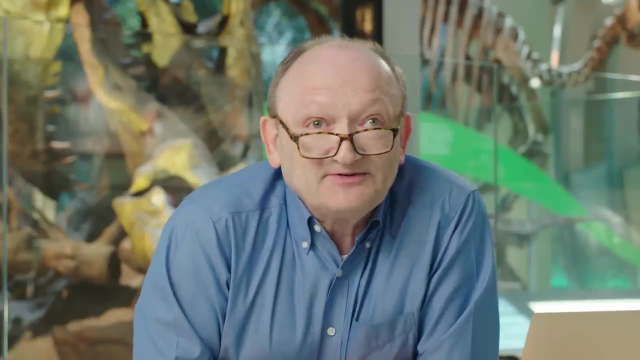 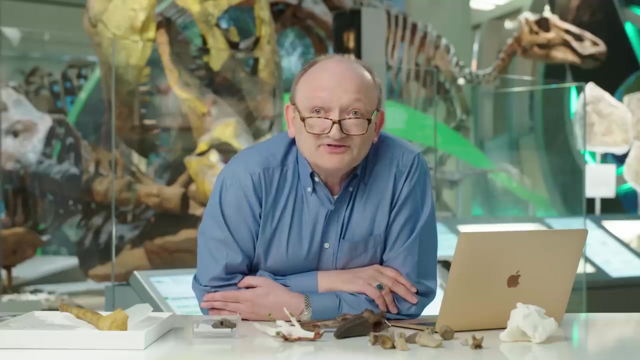 66 million years ago, and, of course, their descendants, birds, who are also technically dinosaurs. to the present day, We don't know much about individual dinosaurs' lifespan. In the case of the T rex, we have found now that the oldest known and largest T rex was only about 30 years. 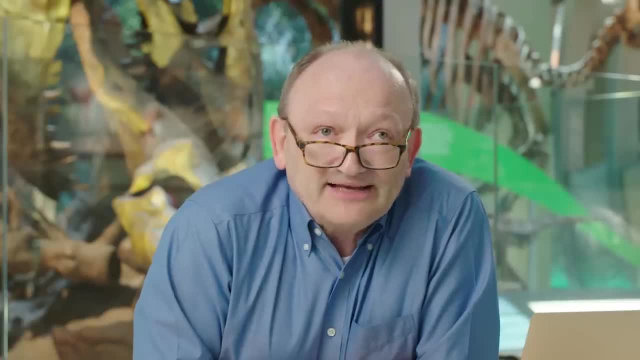 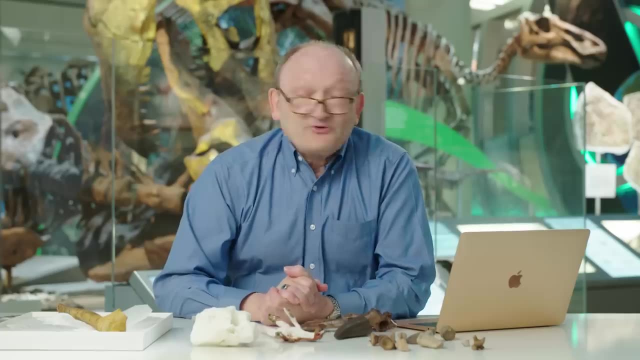 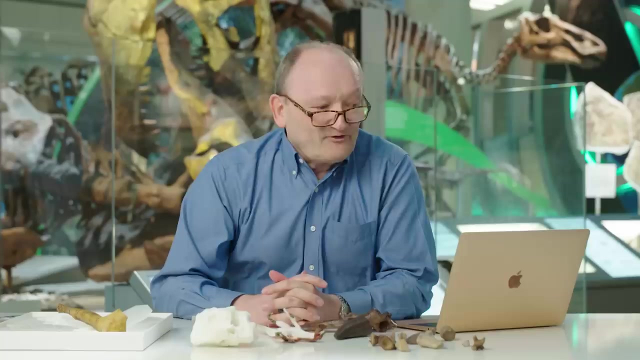 old when it died. These dinosaurs grew apparently at an amazing pace early on and sort of died young and left in some cases a good-looking corpse. So those are all the questions for today. I really enjoyed seeing all of them and seeing the level of interest in dinosaurs out there. Thank you for. 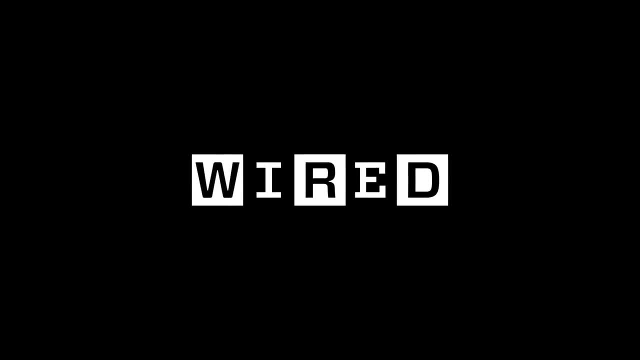 watching. Thank you for watching Dinosaur Support.